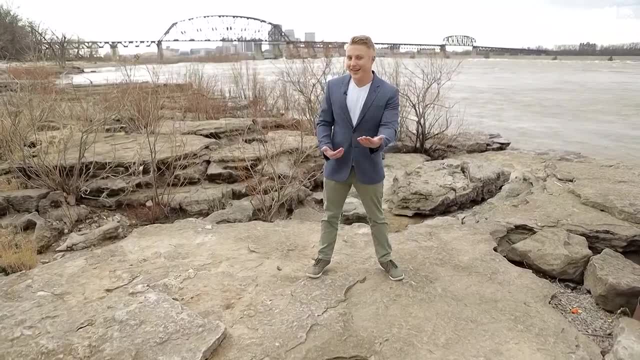 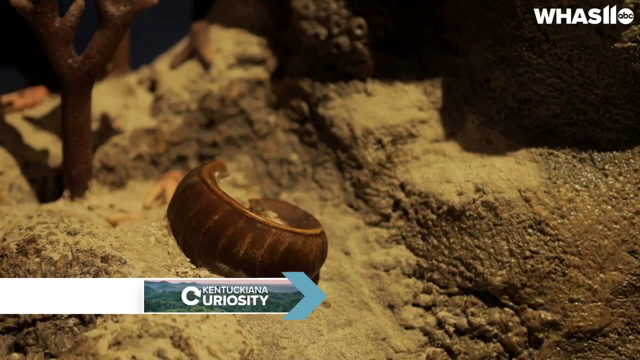 North America to hunt for fossils. And don't take my word for it, take an expert's. My name is Alan Goldstein, I'm interpretive naturalist at the Falls of Ohio State Park And I hate boasting, but I've never met a rock. I couldn't. 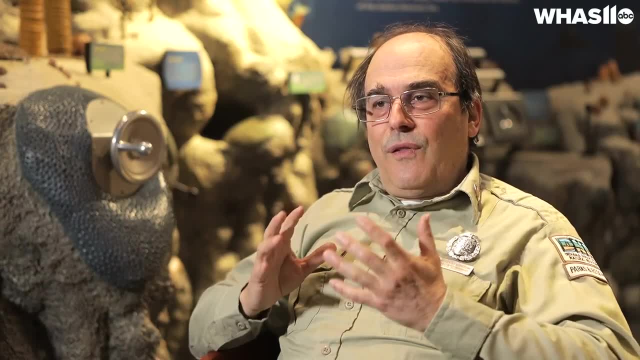 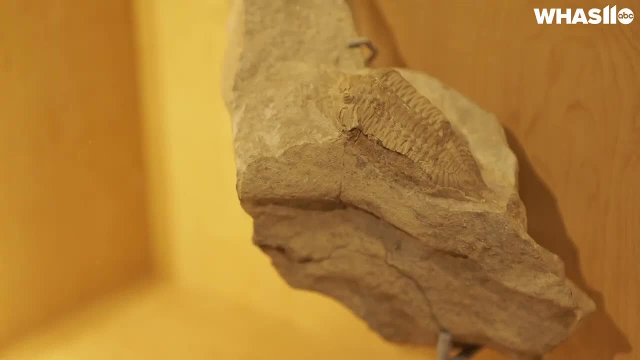 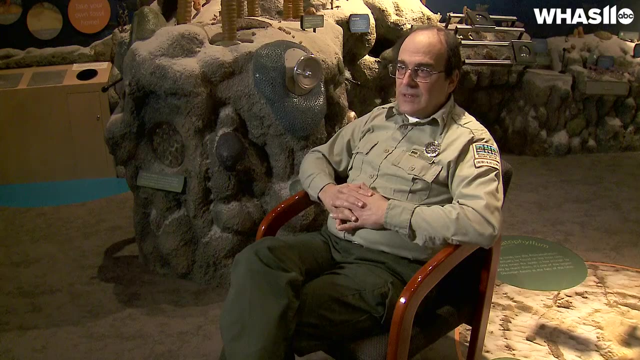 identify. There are very few places in the country that have a fossil legacy as diverse and as rich as we have in the Louisville metropolitan area. you, The fossils here, go back millions of years and you know what we're looking at in the Louisville area. primarily is marine animals. That's the dominant. 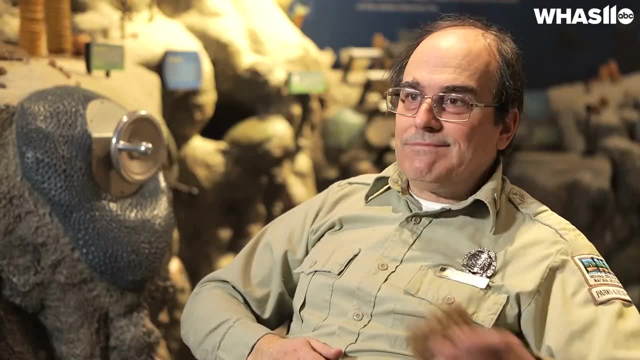 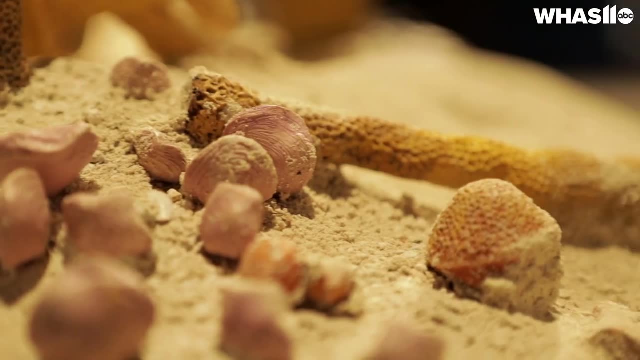 fossil category and it might include something like corals, It might include something like trilobites, It might be brachiopod shells. Brachiopods is the Kentucky State fossil, An animal called a ciloli which is one of these things. 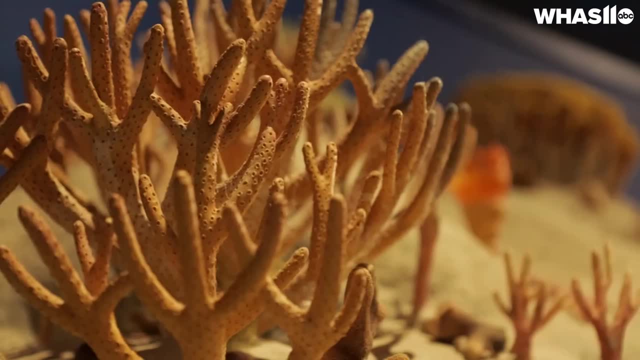 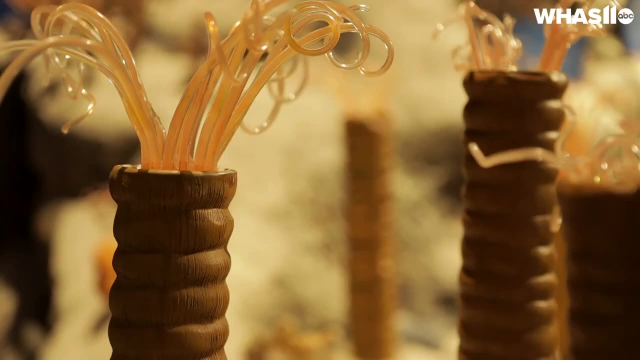 behind us looks like a flower. There's a lot of different things you're going to find here that are things you would expect to see in the Bahamas or the Great Barrier Reef or the Caribbean or something like that. I think that people 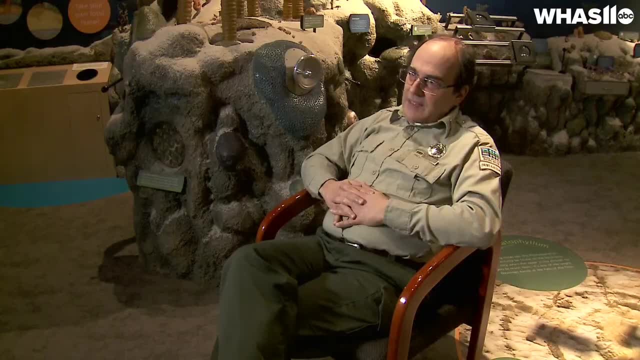 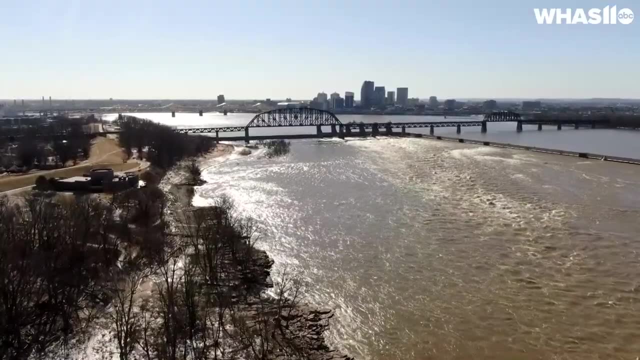 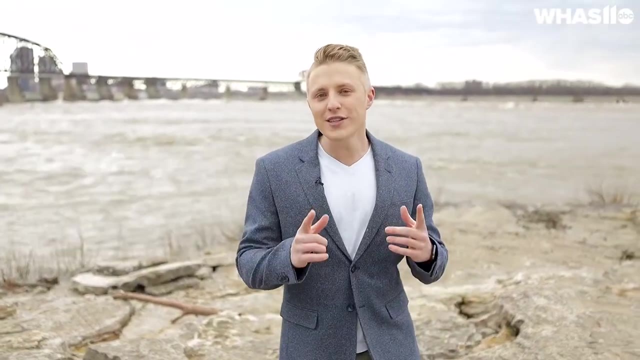 need to have an appreciation of science, because it is science that makes to me life interesting, you know, because there's a story behind everything. Finding fossils doesn't just add cool keepsakes to our collections, and it actually doesn't just tell us what our home used to look like. It also tells us 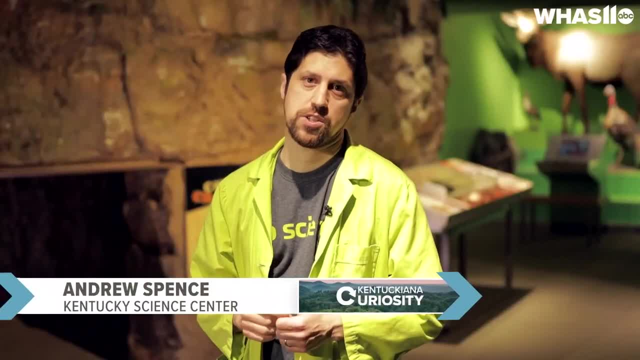 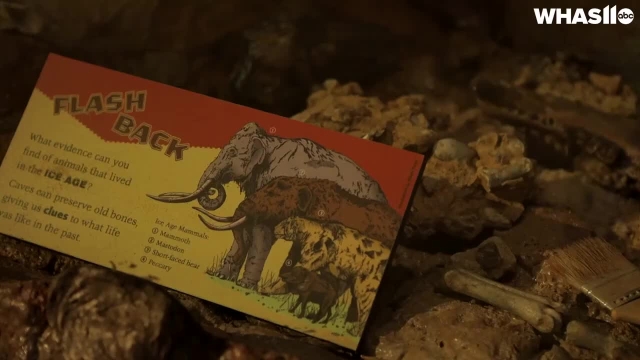 why our home looks the way it does now. Hi there, I'm scientist Andrew here at the Kentucky Science Center and I'm by our cave exhibit on the second floor in the world around us. I also have with me is this large geological map of Kentucky that shows all the different rock types that 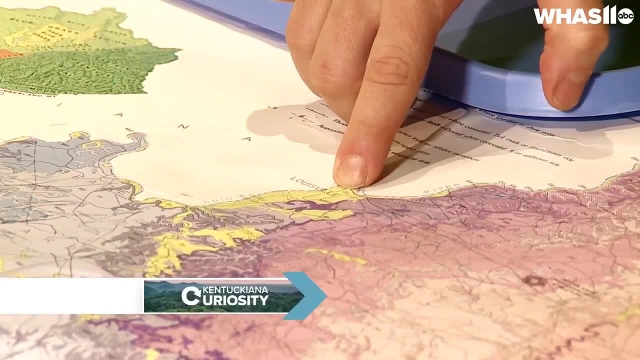 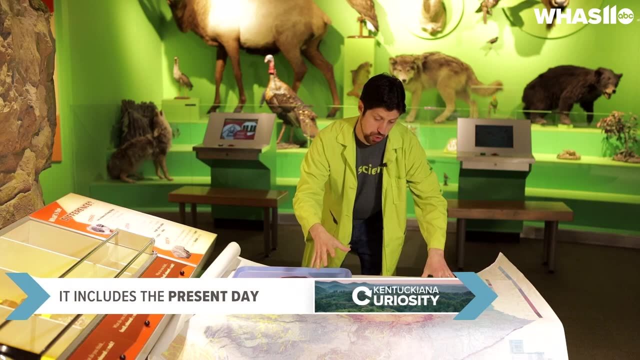 are visible on the surface. Now we're here in Louisville, among the quaternary glacial deposits here in the city of Louisville, but what I want to talk about today is the bluegrass region. So, as you can see, there is a big pink-purple circle. 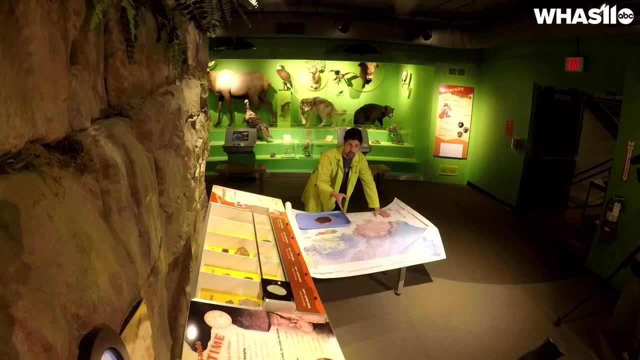 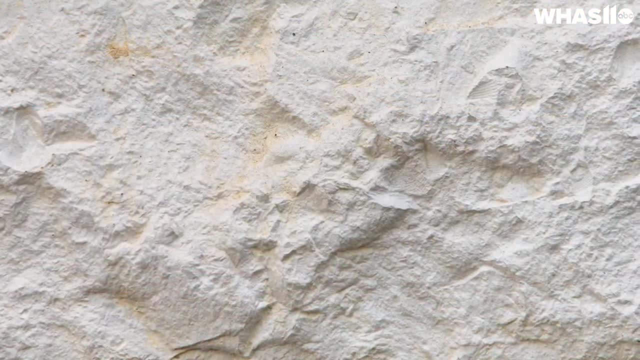 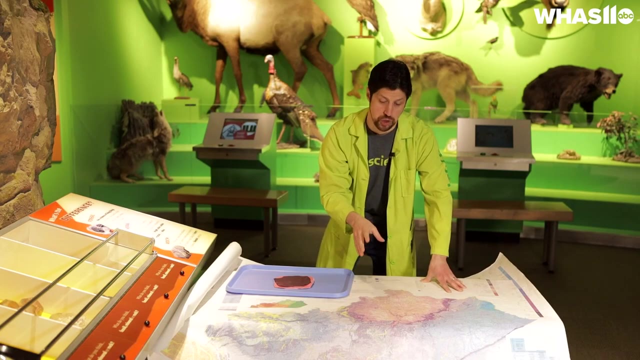 central north part of the state of Kentucky. That's the bluegrass region, known for bourbon, horses, rolling fields, and that's all because of the limestones that are on the surface. The bluegrass region of Kentucky is primarily made of rocks of three different geological periods. You have the Ordovician. that's